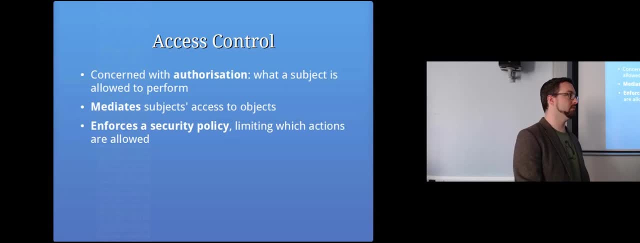 So the stuff from last week about how do you know someone is who they say they are. you need to do that first. Once you know that that person is who they say they are, now you can start to enforce access controls. So I can say: okay, yeah, so Chris, come. 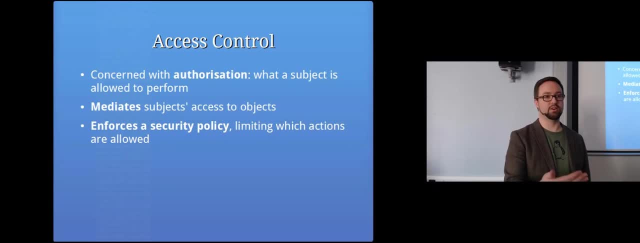 Chris tries to enter a room. for example, you show your badge. check. the photo is the same. So, okay, you are authenticated. I'm convinced that you're. that you're Chris, Then I might look at the list of people allowed in the room And if your name's on that list, then you're allowed in. 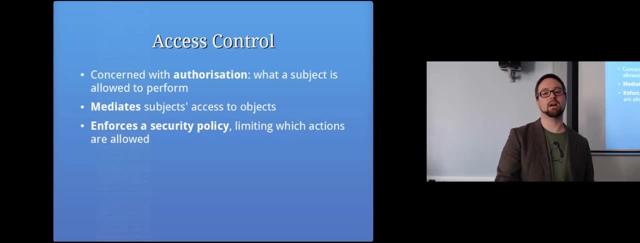 So that first step is authentication, checking who you are, And then access control is the authorization step, where we actually check what you're authorized to do. And the important thing is this: mediates subjects access to objects. So subject is just the person or the thing doing something, So in a computer system it might be the program that's running. 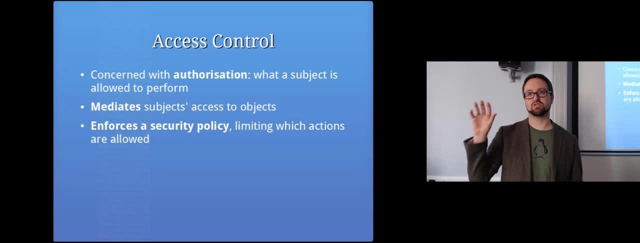 So that process is the subject of the access control. it's trying to do something, And when we're making access control decisions, it's: what is that subject allowed to access? Is that subject allowed to access this object? And objects are just mostly static resources and files. 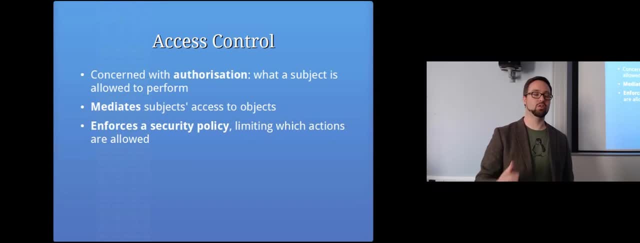 But also if a- you can also say an- object- might also be a process, because if a process is trying to access another process, in that situation the process that's acting, you would say, is the subject, and the process they're trying to connect to is the object. 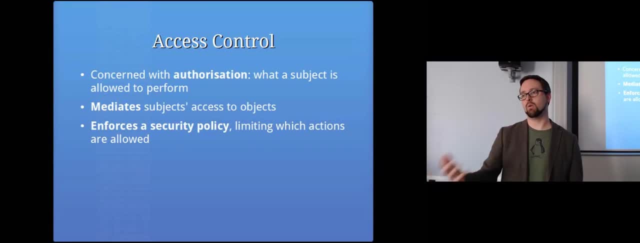 And also if you're trying to access the network, that might also be referred to in those terms as well. But it's all about enforcing a security policy. So we need some policies, some rules that states who's allowed to do what, And then we're going to enforce that with our access controls. 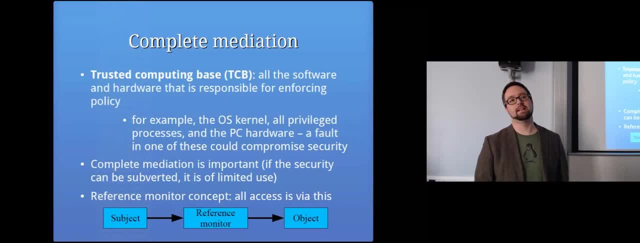 So we're aiming for complete mediation, which means that we really want the security to work and the program shouldn't just be able to access some other program to get the files that they want to access. There has to be a consistent way that the security is enforced. 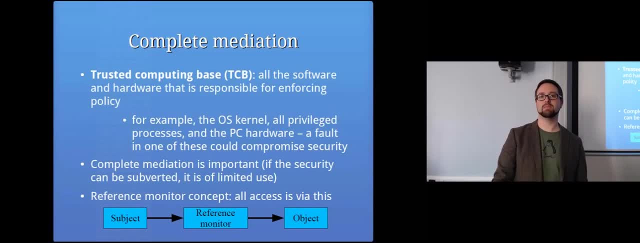 So, for example, if I was the person standing at the door checking name badges, are you allowed in this room? If there was another door at the back of the building and no one was guarding that, that would fail the complete mediation test right. So that would be a bad security design because someone just come in through the other door. 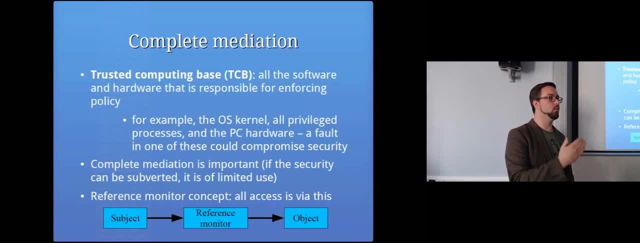 So, in order to work, we need to actually have just like one way of accessing a resource, And we need to be able to carefully define how that behaves, And one of the ways that we are sure that it's going to work is by thinking about the trusted computing base. 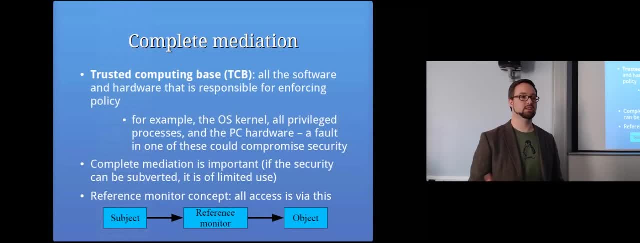 So trusted computing base, the TCB, is basically a term that represents all of the software and hardware and all of the parts and pieces that go together to enforce the policy. So if we're talking about like a Linux or Windows system, for example, that's basically most of the operating system. So let's just say Linux, for example the kernel, every. 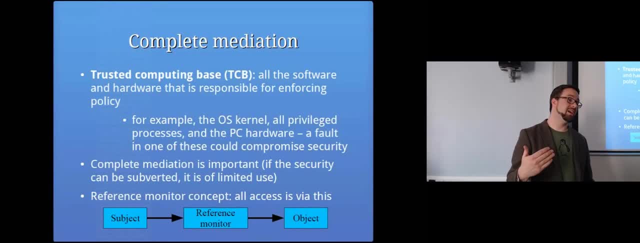 process that is running on that system is root Basically, whatever login programs that are and all those sorts of things. that's all part of the trusted computing base because if there are any vulnerabilities in any of that stuff, the security is all going to break. So that you know, the security at the kernel is particularly important, that it is enforcing security in the correct way. 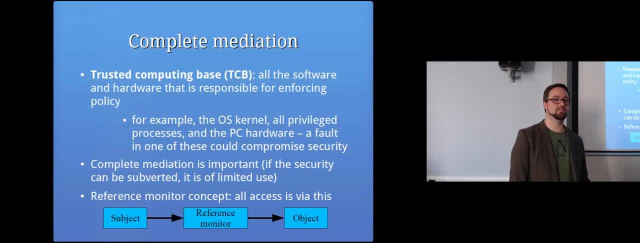 So yeah, even hardware. so there's a news item- I don't know if you've heard from this week or some news item- very clever exploit where basically by flipping bits in memory in on a certain type of hardware, it's possible to basically corrupt different set of. 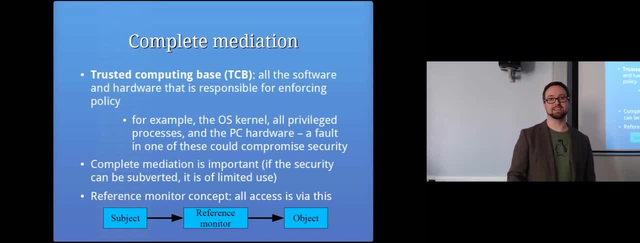 memory, which can result in privilege escalation in in Linux. basically, I mean, it's it's incredibly, it's incredibly clever, but so hardware also comes into it. so all these things go together to actually enforce the security if we can. if the person can basically avoid the security controls, then where you know, 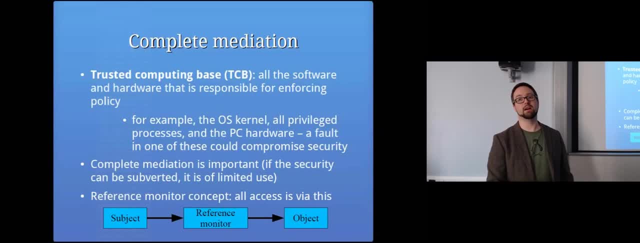 it's not good. it's another example that might be email in an organization. if you have this really clever access control policy that specifies which people within an organization are like that are allowed to access certain files, say, it's a really difficult system to use. people might 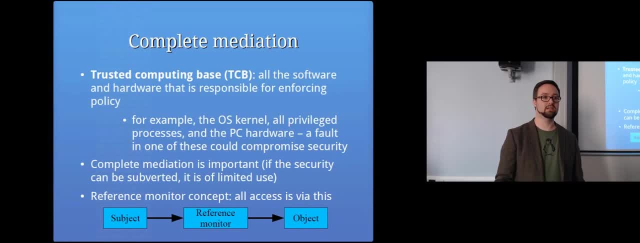 send up emailing all the files they need back and forth between each other, and that's that's horrible, right, that's the worst thing for security, because now they're going around the thing that's supposed to keep those files controlled and who can access them as soon as people start just like ignoring that and 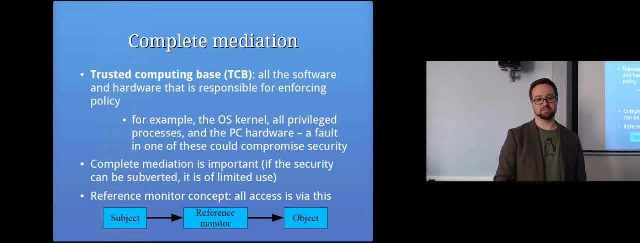 emailing things to each other, then you know that security systems failing, so ideally it shouldn't be possible to not access things through our security system. reference monitor is basically a concept, that that there is this thing that you use to access the files. so again on Linux, it's the kernel. 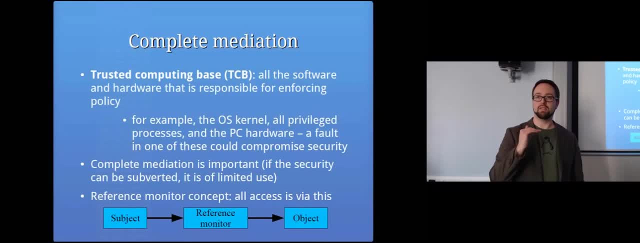 every time you go to access a file, that request is via a system call. so program says to the kernel: hey, give me this file. and the kernel says let me just check if that's okay and then if it is okay it gives the basically gives access to that file to that program. so every single access to a file. 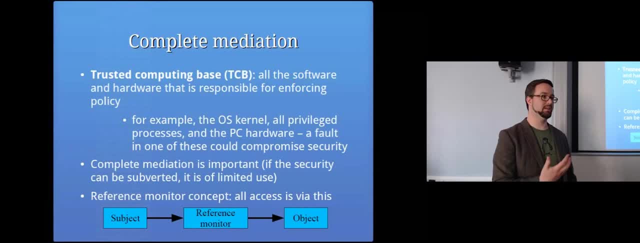 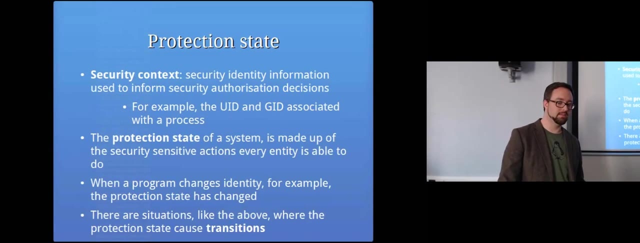 goes via the kernel and a specific set of you know the security subsystem within the kernel. so that's basically a reference monitor where you have something that mediates access to everything- the protection state against more terminology- and is like the- this complete state that the computer is in in 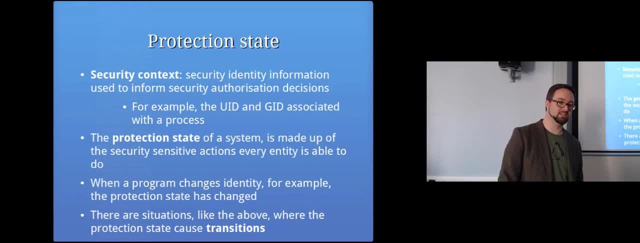 terms of you know all of the processes and all the identity associated with them, or security context is the identity or the information assigned to each subject that is used to inform the access decisions. so if we were talking about this exact the- it's XAT, the people's name badges- knows David allowed. 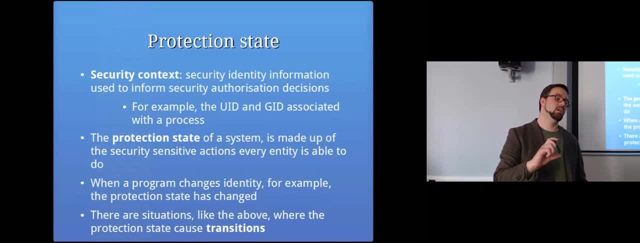 into this rain crisp on the room in my life in the room. The security context in that situation is: if I've checked your name badges already, the security context is the information written on your name badge. That's the information the person at the door is using to make that decision. 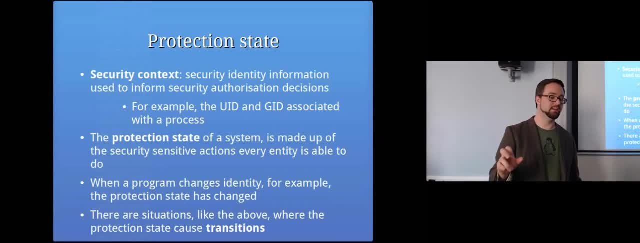 So on a Linux system, that's the UID and the GID and other security information that is associated with each of those processes. So you guys are processors on a computer and you're trying to access something. look at your name badge. What does your UID say? 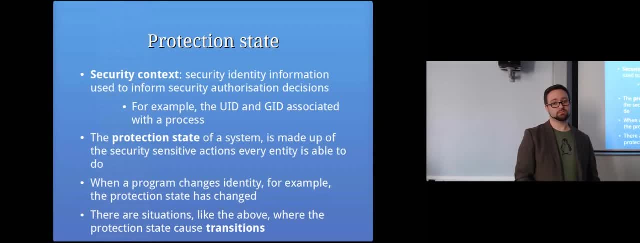 Is that user allowed to access it? The stuff happens on a computer, though, where you might change your name badge, So you might. maybe, I don't know, maybe Umar has permission to sometimes act on Taz's behalf, So Taz may have in the past said: yeah, it's fine, you can access that file for me or go. 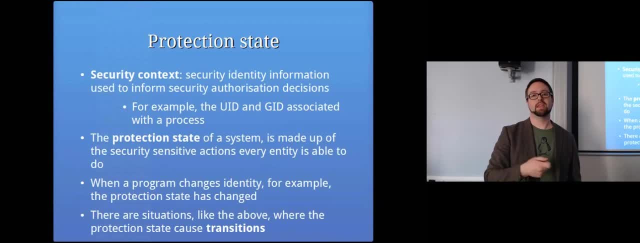 into the room for me. Here's a name badge And then it's a piece of paper that says you're allowed to use my name badge or something, And then you might put Taz's name badge over the top of your name badge and in that situation, 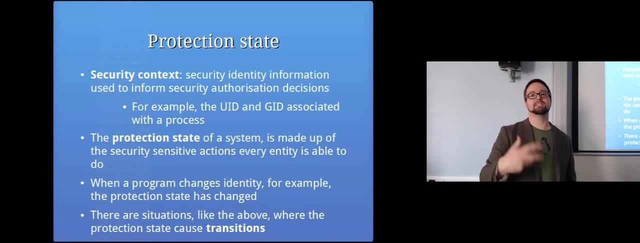 you've assumed that identity and that's okay. but the act of doing that is a transition in the protection state of the system, because things have now changed and now you're acting with a different set of permissions. So it's really important on the computer system to clearly define what kinds of concrete 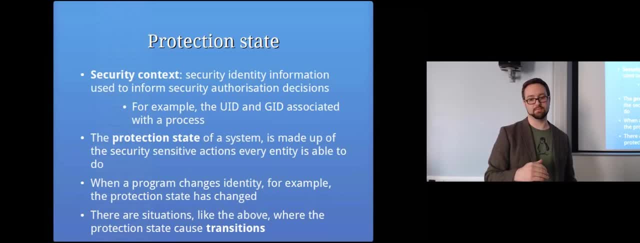 security context changes are allowed. How are those transitions? what are you allowed to do? how are you allowed to change it? That needs to be really tightly controlled, obviously, and it might be that you need to actually go up to someone else and say: can you swap over my name badge? 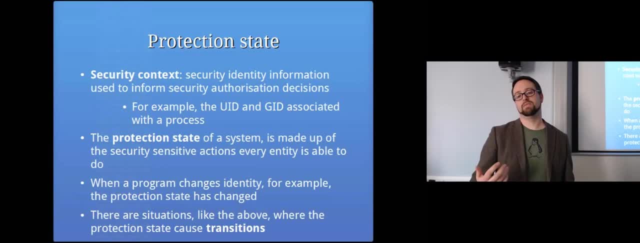 You shouldn't just be able to randomly change your own name badge. So again, that's an analogy for on a computer where you might change your UID so that you can do something that you're not normally allowed to do. So there are various ways you can do that on a Unix system, and that needs to be very 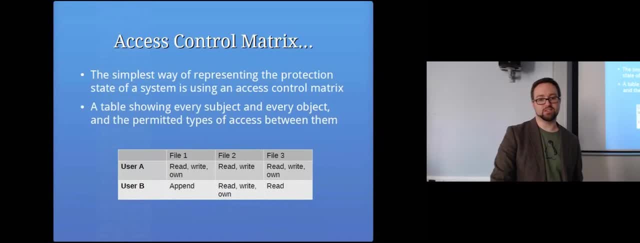 tightly controlled. So an access control matrix is the simplest way of describing a security state And basically it's just a massive table explaining every single access permission that is possible and whether it's allowed. So in this case we have user A, user B, a list of all the different, every single user. 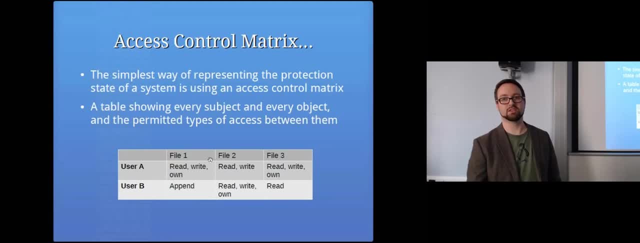 is on this table and every single resource that's on the computer or in the room or whatever, is all laid out in this table. And then, for each of these cells, is whether or not that subject is allowed to access to that object and in what ways. 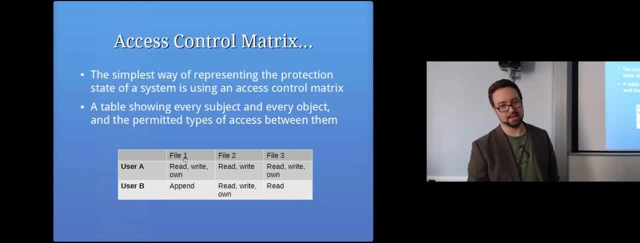 So in this example here user A is allowed to read and write to file one, And actually that user owns that file, So they're allowed to change permissions and things for that file, Whereas user B is not allowed to read or write to the file, they're only allowed to append. 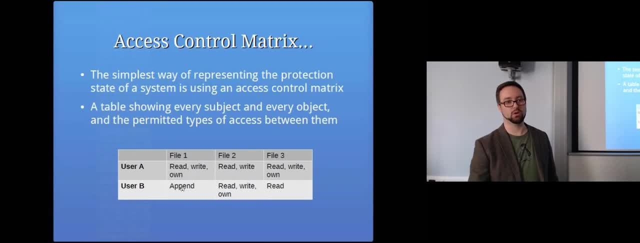 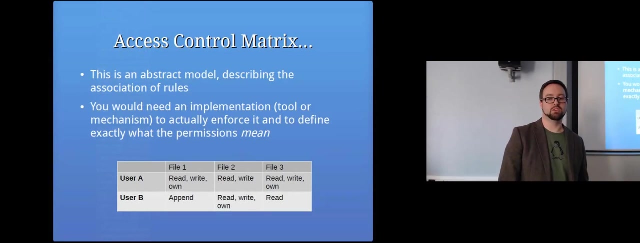 to the file So they can just stick something at the end of it. They can't access what is inside the file or change what's inside the file, and so on. So this is an access control matrix. But this is basically an abstract way of thinking about things, because in reality you would. 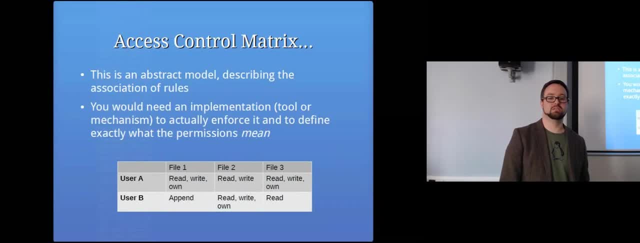 never use this. You would never use this system because just you know how many people you know. this table is just going to be massive. once you've got 100 files you know and 10 users, It just becomes unmanageable. 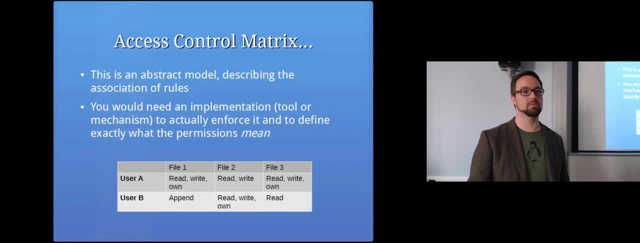 So that's not the way that we store information about security, but it is one way of thinking about it. So we actually need some kind of implementation to actually enforce this. And also you need to define: what does this mean? What does reading mean? 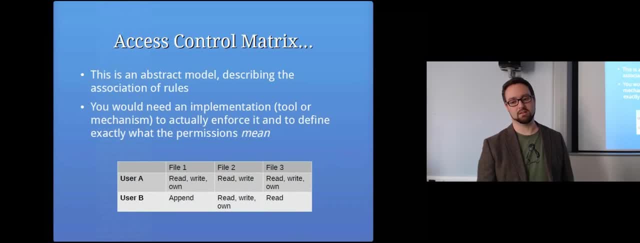 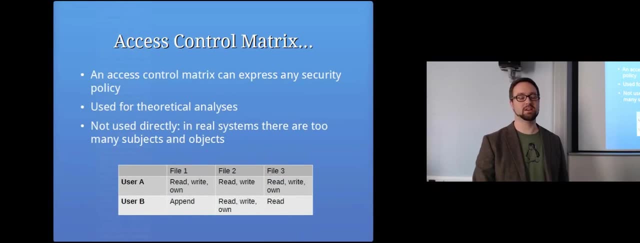 You know what does writing mean And owning it. What does owning give you the ability to do? But the nice thing about an access control matrix- this big table- is you can use it to express any policy. If you've got this massive table, you can express anything this way: 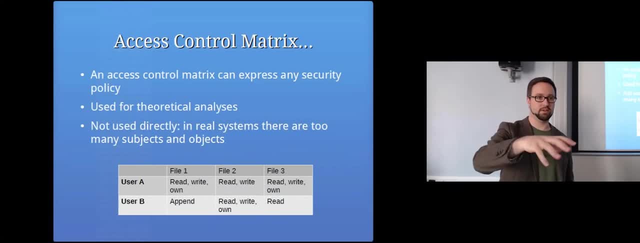 So I could say that you know, you three are allowed to access these files and you guys are allowed to access this and these ways and everything like that. But yeah, it's mostly used for theoretical analysis and things, so it's not actually. 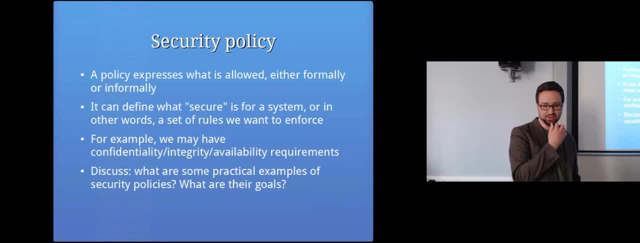 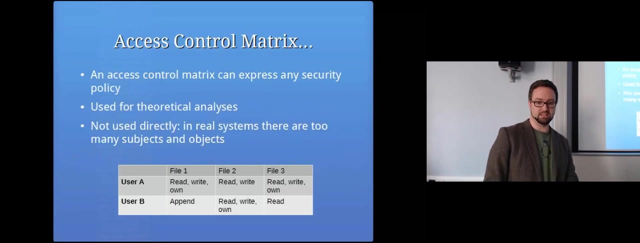 used in real life, But we will come back to that in order to explain. you know different types of security systems. So a policy defines what's allowed, So that can either be formally or informally. So a formal policy might literally be, you know, like this: 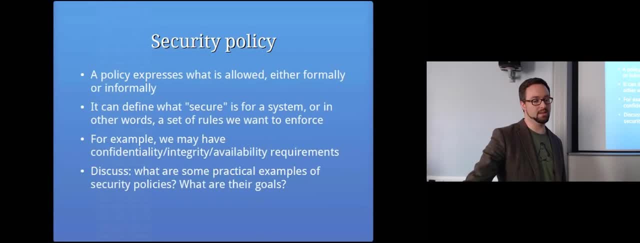 This is what these users are exactly about to do. An informal policy might be more like in a business context, the sorts of things that you're supposed to do And you know, not specifically specified. Okay, If it's just written in English, it can be, you know, a bit ambiguous. 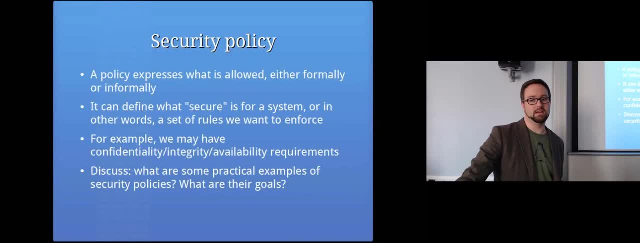 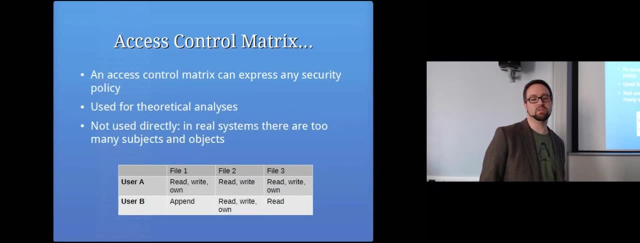 But a security policy basically defines what's secure and what are the rules that we're trying to enforce. So if this is our policy, this access control matrix here, if user B finds a way to write to file one, they've managed to subvert our security system and we're in an insecure state. 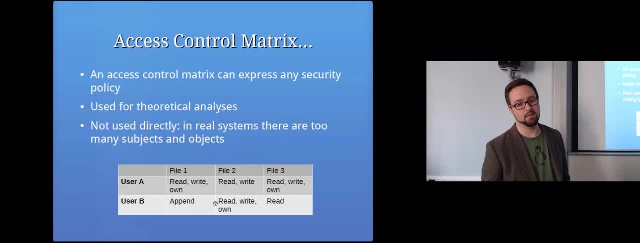 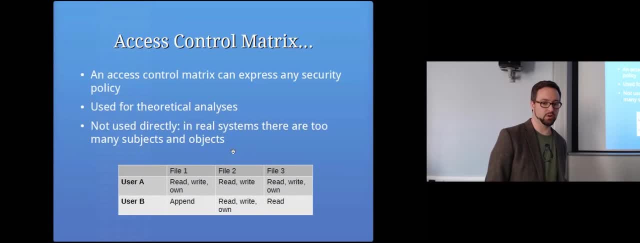 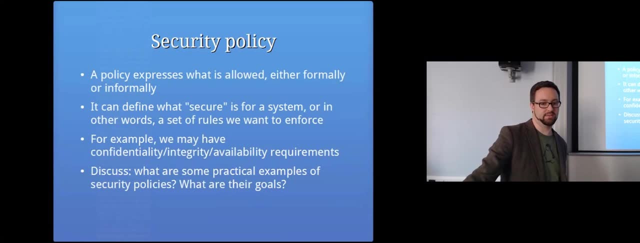 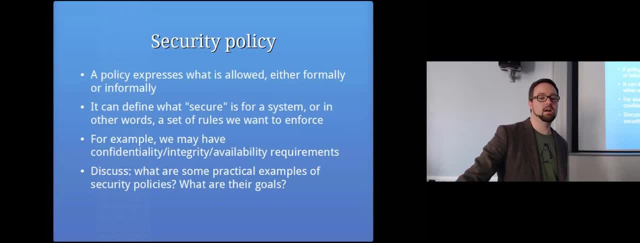 So, again thinking about those basic concepts in security, um, you know, uh, do we want people to be able to read certain information? We are they like to change it and, you know, is it available to them? basically, Um, can you guys think of practical example? 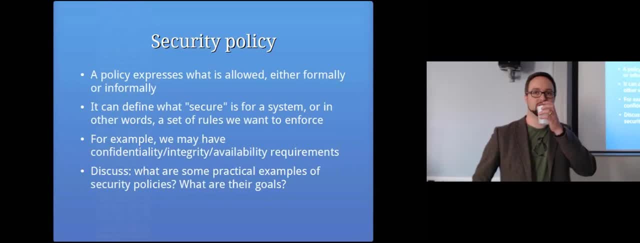 Could you do a very clear, elegant description here and then you so basically it might, in Examples of a security policy, just anything, just to You know. we all know what the terms mean. yeah, Yeah, Yeah. so you will. often organizations will Say whether certain resources are supposed to be publicly available, and a lot of time. 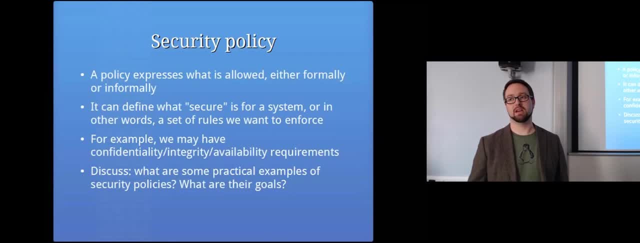 There's a lot of information that shouldn't be available to the public and I don't know. can you think of an example of when information that we wouldn't want to share? That's a reason. but yeah, finances, finance is a good answer. Sorry, Company policies, yes, you know some of that stuff You don't really want everyone to say. 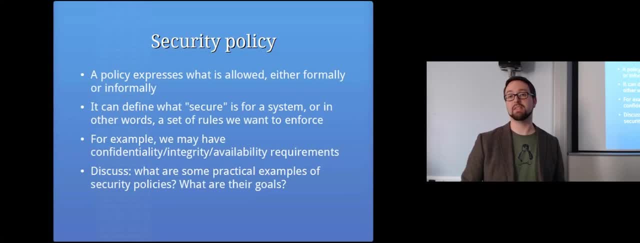 So, yeah, there's all sorts of reasons why you don't want stuff to be available, And in that case, Are we talking about confidentiality, integrity or availability? Yeah, so it's about what someone has, you know, the ability to read, so that's confidentiality. If we're talking about whether someone can change something, we're talking about integrity, and whether it's something that's available is availability. 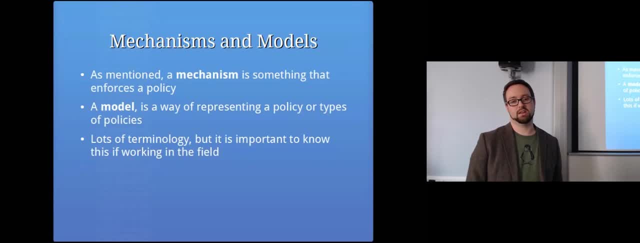 Yeah, okay, So you know, as, as we've discussed, a mechanism is something that reinforces a policy, and So, for example, a firewall is a mechanism. right, it's a thing that does something. a Model is a way of representing a policy or types of policies, And so we're starting to get a bit abstract. So, a way of 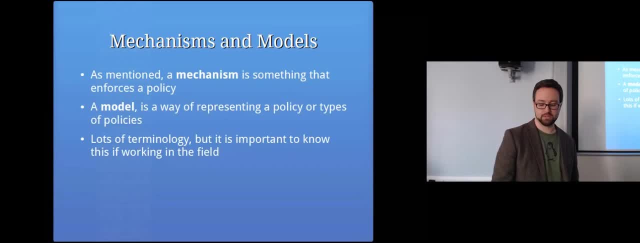 Representing the kinds of rules, So, for example, the You know this access control matrix. That's like a security model and Again we are I'm introducing quite a lot terminology, But this is really important, especially if you end up working on the defensive side of security. 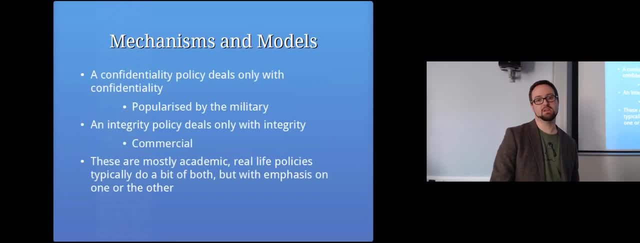 You know, or any type of security. it is important to understand this stuff. So, Okay, I just said all this. the confidentiality deals with sorry. confidentiality policy deals only with confidentiality. So there are types of security systems that the military use, for example, Where the most important thing to them is that things they remain confident, confidential. So there are security systems. 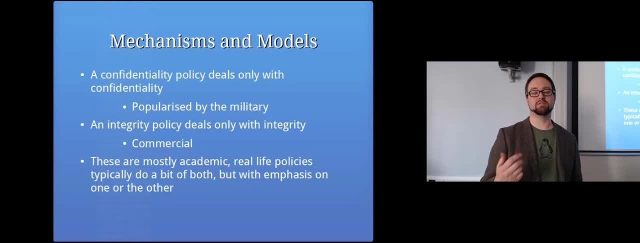 They have. that will basically Won't stop someone from altering information. as long as they can't see the stuff They're not allowed to say, That's like the most important thing to them. an integrity policy deals only with integrity. They're really. it doesn't matter what people can see, but it's super important that no one can alter this information. 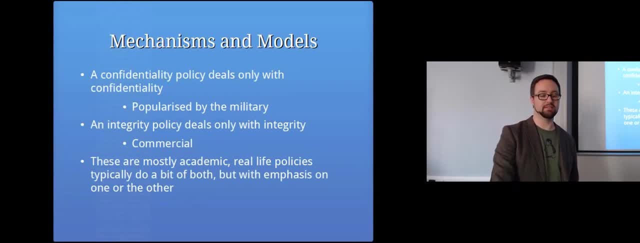 That's like the most important goal for us, and that is often the case in like a commercial setting. But in reality- as like you can probably guess what I'm saying this- Most people want a bit of confidentiality and integrity, So we have like a mixed model. 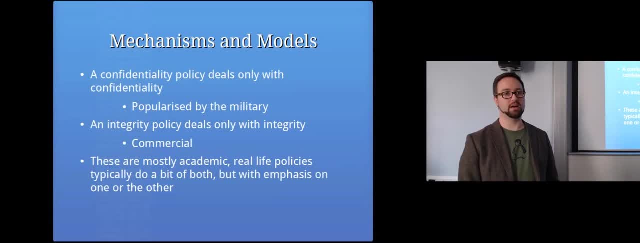 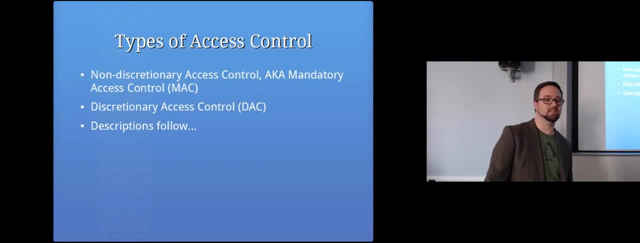 So real life policies do a bit of both, You know, but there usually is an emphasis on one or another. so Some types of access control. So these are access control models. There's non discretionary access control, which is also known as mandatory access access control, and there's discretionary access control. 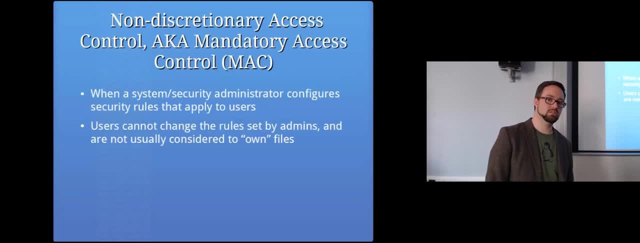 Those are the two big ones, So I'm going to talk about those. so, non discretionary access control, Or mandatory access control, It's one of those areas where the people don't agree with the terminology that you should be using. basically, mandatory access control is when, as a system, 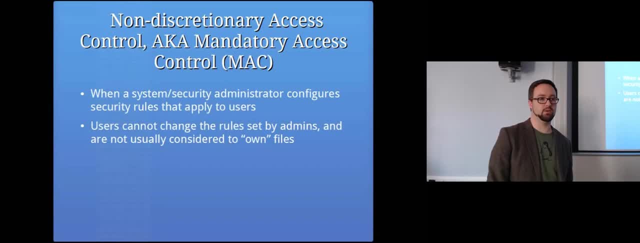 Administrator or security administrator gets to configure the security role rules, and that applies to everyone. So if I, for example, Had this list of who's allowed, Hang on, Let's. let's adjust the analogy so it works better and say: we've got a room and 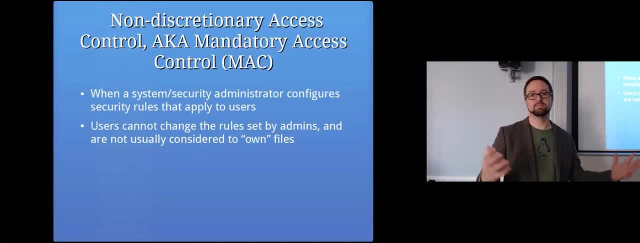 This analogy is really boring. got filing cabinets and there's certain filing cabinets have different types of information in them, So, for example, one might be for finances, one might be for use Personnel information, right, and all of you guys have name badges and you're allowed in the room. 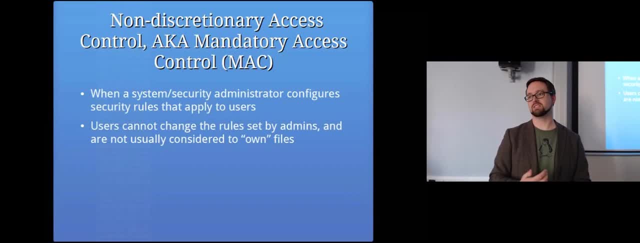 But someone standing next to these two filing cabinets and just checking that you're allowed to access that filing cabinet. It's not a very good analogy, but we'll go with it. So it's like it's almost not even analogy. It's like what's happening on a computer. So 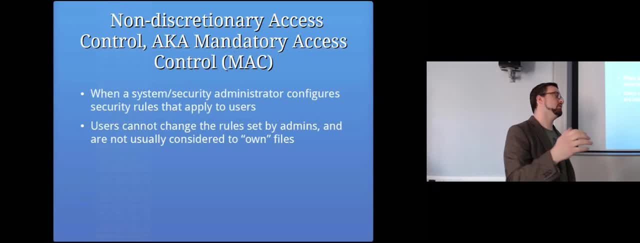 okay, so that's what's happening, and if I Get to write all the rules about That information, then we've got a mandatory access control system. So you guys have no say over what you're allowed to access, because I've labeled all of the files in these and filing cabinets with 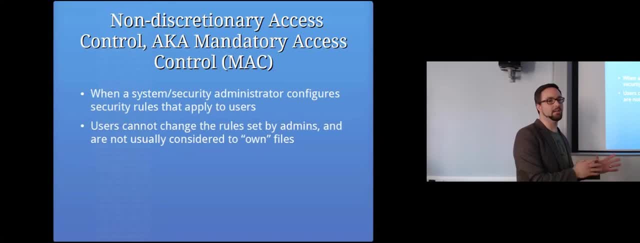 information that says this file Is about personnel information, this file is about You know all the. everything in this folder is about finances. and then I've written on your name tags- You know your name. and then on my little piece of paper that no one, none of you, gets touch. 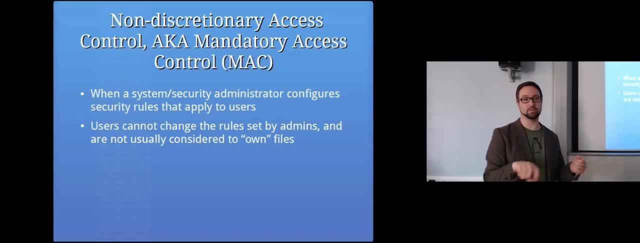 It says list of names and whether or not you're allowed to access certain things. right, That's managed access control. You've got no choice. You can't change any of the security policies. you are subject to them and you have to. basically, you've got no ownership over any of those files either. you just have access to them and 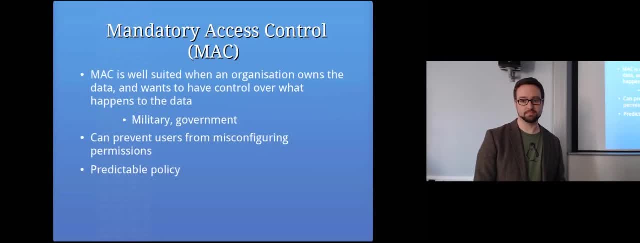 The rules specify where you are to do so. that is mandatory access control. So it works well when the organization owns all of the data. So all the information is owned by the organization, and well, I wanted to keep my tight control over what you're allowed to do. 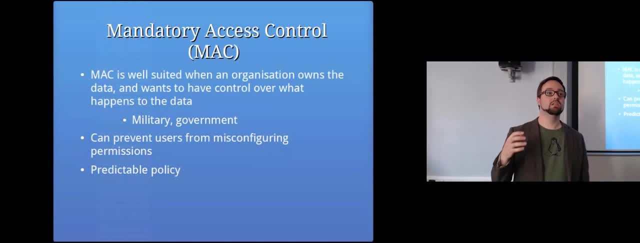 So, for example, in the military or government, as often the case. so I Really know that you're only supposed to access certain stuff and it can Prevent the problem where you guys, if you were allowed to change who's allowed to access what and you made a mistake, you might. 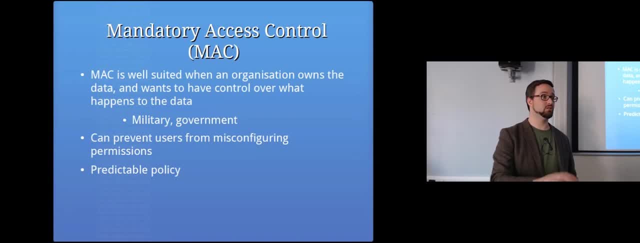 Accidentally end up doing something that you don't mean to do, so that stops you from making mistakes, And it's really predictable. for me, being the person that's in control of all these files and everything, I know what's going to happen. It's quite straightforward and 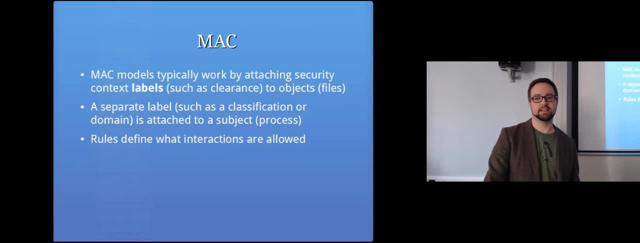 Usually the way that works on a computer is you. you literally attach a security context label to an object. So I attach some information to each individual file on the computer And also I attach a separate label to every single running Process or every user on a system, and then there are rules that say what's allowed to happen. 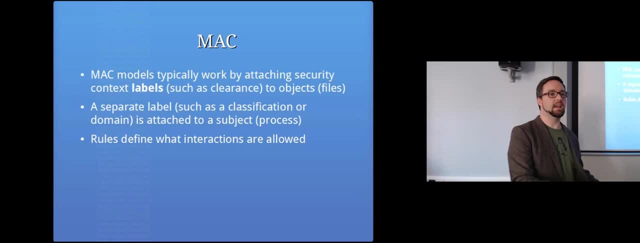 So it's literally exactly an analogy is not so bad. So in in this example, if I had certain printouts and I put a sticky note on it that said: you know, Is this a per is? is this specific file a You know, personnel information or finance information? and then I look up on my name and I look, you know. 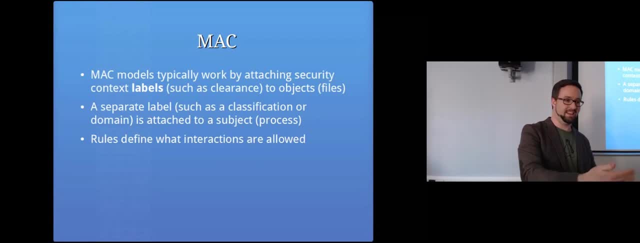 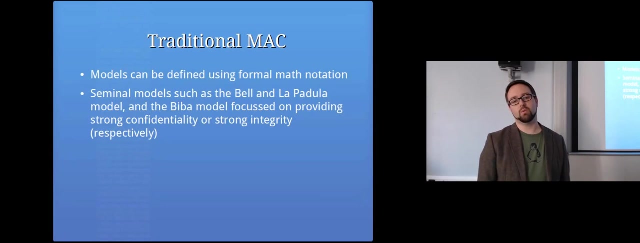 Is Chris allowed to access finances? Say yes, so yeah, okay, so you, you can access it. That's what happens on a computer, basically. So so yeah, there's rules that define what's that happen. Some ways of modeling traditional managed access controls is using like formal. 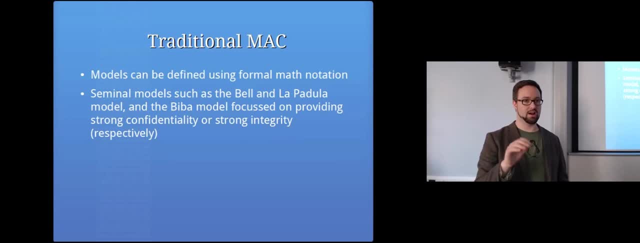 Math. so there's like actual, like a notation that describes exactly how this model works, and the seminal models are very important. traditional lab papers and Models that have been proposed, Such as bell and Formatula model, which is focused entirely on confidentiality, and the Bible model, which is 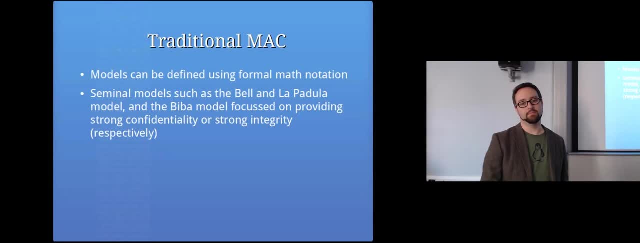 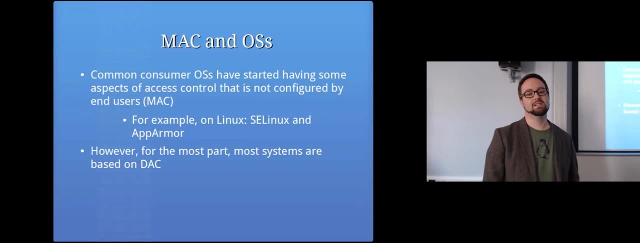 Entirely about strong integrity, But it's still possible to心 rav4 starting to become the case where there are some security features in things. you know, consumer operating systems like Windows and Linux, where we can do things like this, where we can define security rules that the users have no say over. so, for example, on Linux, we can use SE Linux and 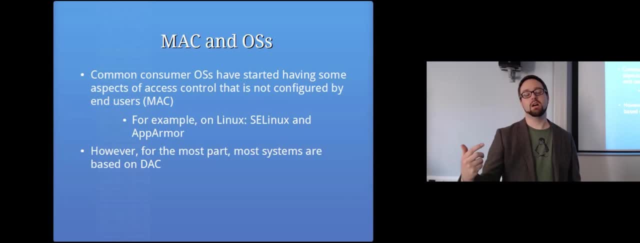 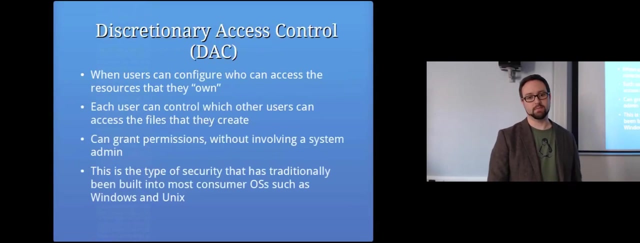 AppArmor and that stuff that we'll look at in the next topic in the module when we start looking at virtualization, sandboxing and things. but for the most part, systems aren't based on what we've just described. right, what I've just described is not the way that most Windows and Linux systems work, so the 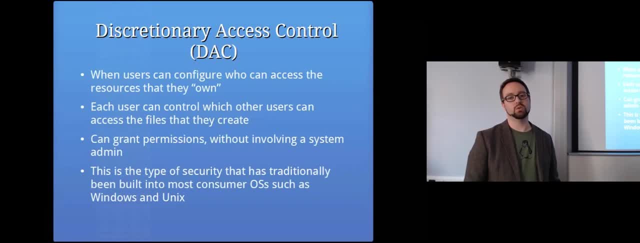 way that they work is by a discretionary access control, which is where users own the files and get to choose who can access them. basically, so in this previous thing, where I'm standing in front of the set of all the files and checking against my set of rules, and that's not exactly how it- 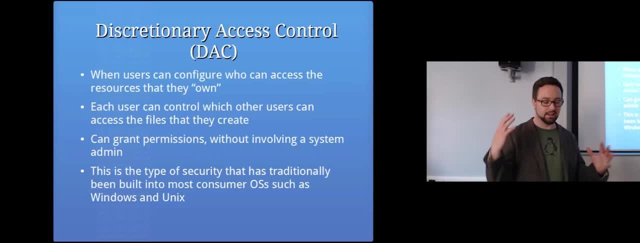 works- I guess my altering my analogy slightly- say: we've got a. each user has their own folder with their own files in it and you get to say who's allowed to access them. so in this situation there might be a list on the front of a particular printout where you get to say who's allowed to access this file. 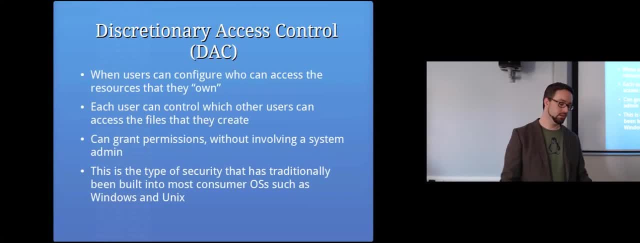 and I might still be standing in front of the the filing cabinets just to check that you're all behaving yourselves. but now you guys get to define what the policy is. so, Chris, you might have, you know, a certain file that you want to share with David. so you might change the rules for that file and say David's. 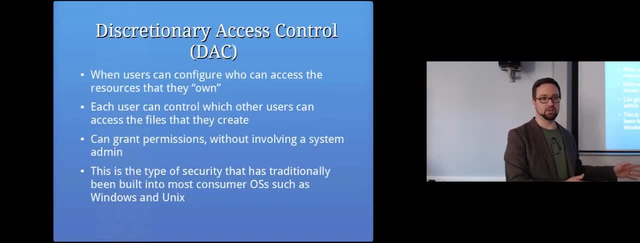 allowed to access this file and obviously I'm standing there and check that you're allowed to access this file and you might change the rules for that. you're only. you get to write on the front, say who's allowed to access it. but now you know, it still might be that Stig can't come along and access that. 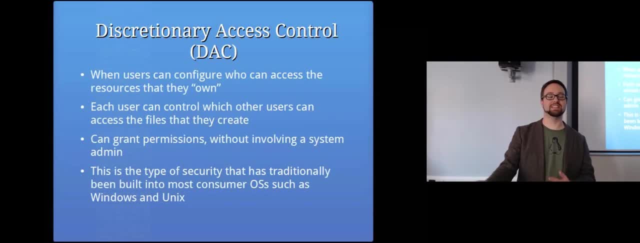 file. sorry, because his name is not on the list of who's allowed to access it. but if David comes along, it's like: yeah, I know that Chris said that you're allowed to access the file, Chris owns the file, and maybe you're even allowed to say: I'm gonna give away ownership of this file to someone else, and then you 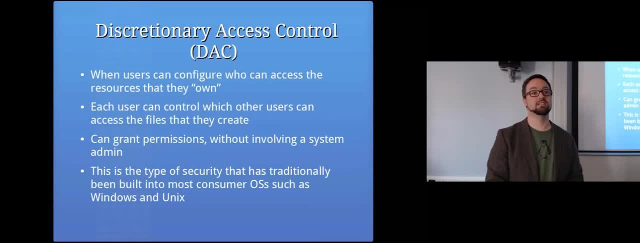 aren't allowed to change those rules anymore. the files now owned by someone else? yeah, yes, yeah, yeah, so you get to specify who's allowed to access the file. yeah, so, like Google Drive, that is a form of access controls. so there's a list of people and what they're allowed to do. on on that. 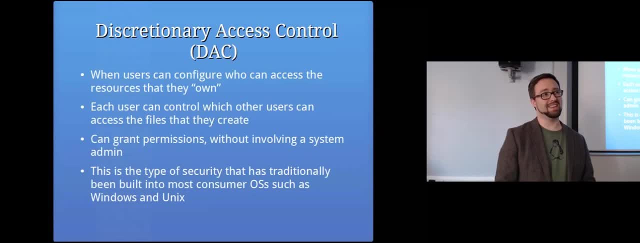 file, and I don't think on Google Drive, though, you can give away ownership of. as far as I'm aware, they can give full edit. yeah, yeah, so on on, like a Windows system or a Linux system, you can give the file away entirely if you want. so you can say yeah. 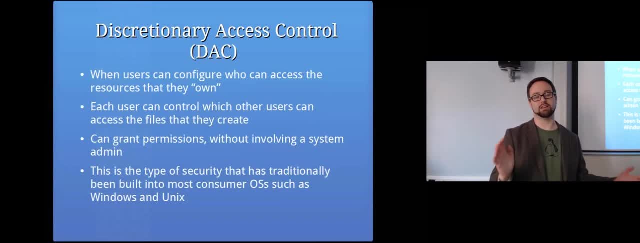 you own this file now and then you've got no longer have any control over the permissions on it. but yes, so there are ways of a user controlling their own files, basically, and you can basically specify what other people are allowed to do. but, as you can imagine, it's a little bit chaotic, right? 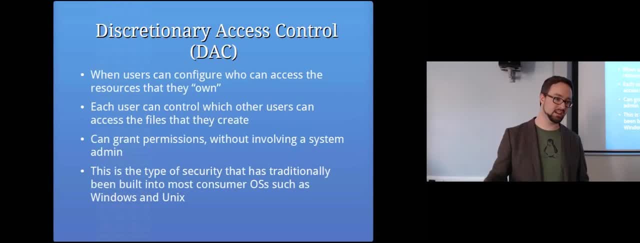 so all it is so many interactions and ways that permissions can change. so if you were an organization like the military, that's not going to suit your needs very well, is it? but for real everyday life it works quite well. I mean it's we get by with it on Linux and Windows. you know we've got by on that. 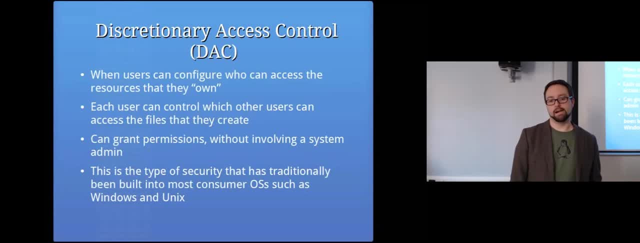 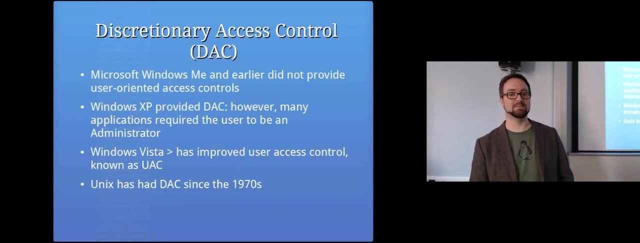 system for a long time. I mean it works, so that's, that's what we're used to using. if you're using older version of Windows, like Windows Millennium Edition- if anyone here can remember that- and earlier, so, like you know, talking about Windows 98,, Windows 95, Windows 3.11- there was no access controls at all. 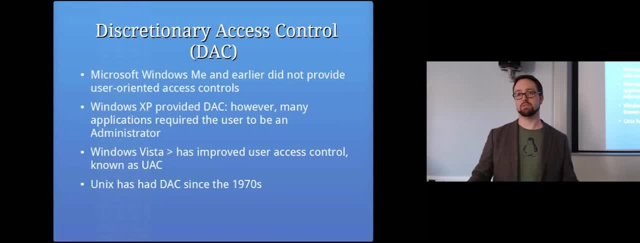 there's literally nothing in place to stop you from accessing each other's files. it was just free-for-all in all senses of the word. there was no controls there at all. you know there's only in Windows NT the server systems where they actually had some form of security actually there for access controls, and Windows XP provides. 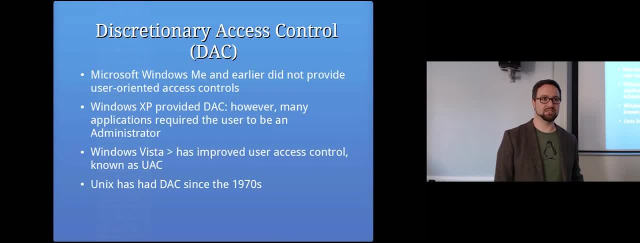 discretion access controls. but almost everyone runs as administrator on Windows XP for practical reasons, because if you don't run as administrator, all the programs complain and crash. but you know, since Windows Vista there is actually user access control is available in Windows and it now your. if you're using Windows, it's good because you can run as, not an. 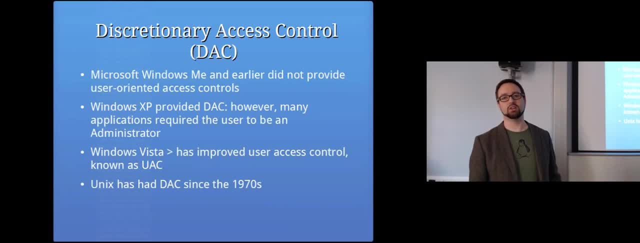 and I'm just talking about MacOS administrator, the phone call from Australia. so, yeah, so now you can actually have a Windows system where you run and you know it's not possible, you know, hopefully make the most maximum Çok gutter than I thought and it was really cool, really helpful for me, for things, yeah, all that we're doing. so it's there's still time to make that one. and you know things that we're really really goodieren- a really goodits sudden call from Australia. so, yeah, yeah, so now you can actually have a Windows system were you run- and you know it's not possible, you know, hopefully it makes it harder, just actually it doesn't make it more difficult, but it's one of those other service options. um, this system which your running, grounded at batwick, you know it's your Need. primarily, this is something that you're gonna have talking to, you know, and if I'm going to ask you 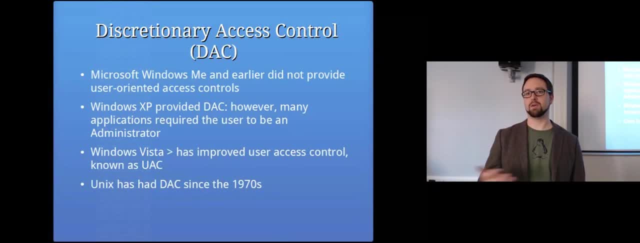 accidentally screw up your whole system or for a security problem to cause a huge, huge impact, but that's something we can talk about again later. unix has had discretionary access control since the 1970s, so all along there's been security in place on the unix system. 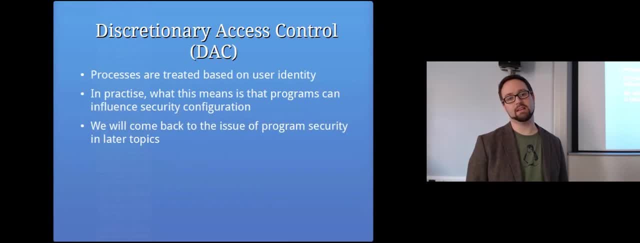 so the way that discretionary access control usually works is: the processes are traded based on user identity. so you know i was talking about name badges. you know we've said this before. hopefully you got- hopefully you're sick of hearing me say it- that the processes on a windows and a 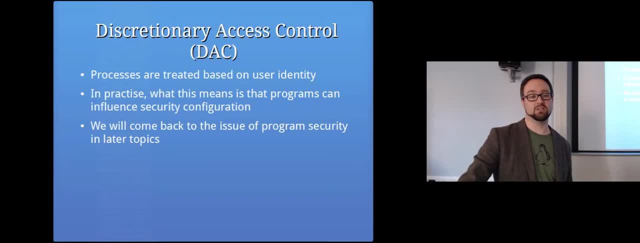 linux system is. most of the security decision is based on who started that program. so what is the user identity associated with that program? in practice, what that means is that programs can influence security configuration. so, um, you know a user. a program can then set permissions on your own files and things like. 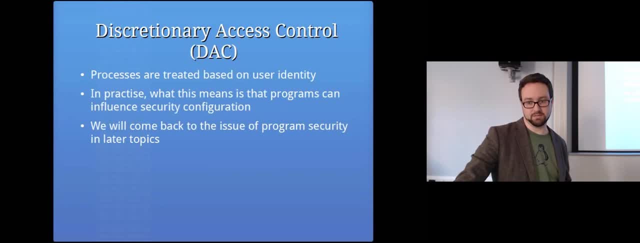 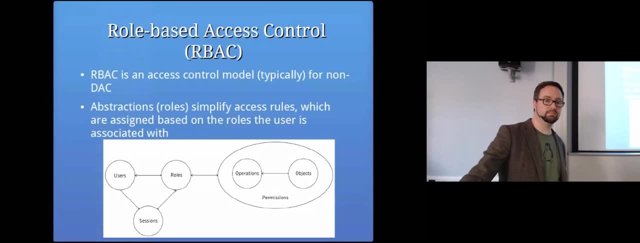 that because the program is running with your permission on that system and we're going to come back to program security throughout the module, really, um, so another kind of access control in addition to role-based discretionary access control- manager access control. one of the main models used to describe access control is role-based access control. 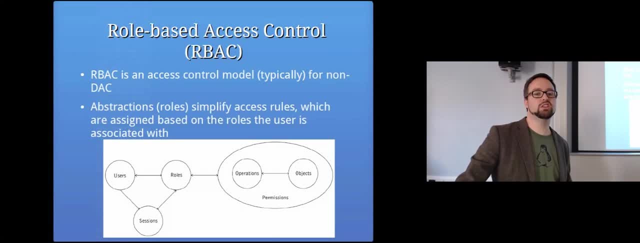 and that's um. usually you'd use for non, non, um, discretionary access control, so kind of a mandatory control usually now basically the. the idea is that if we've got an organization, everyone who has certain roles within the organization should be allowed to do certain things. um, and this is slightly 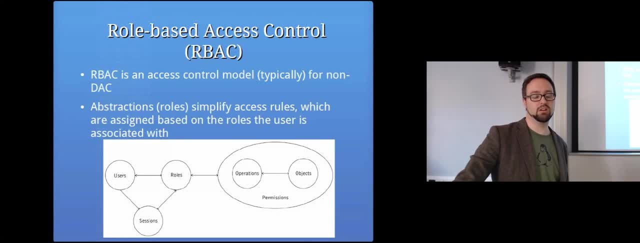 different from groups. um, but it's a similar concept. um, but if we have a um i don't know- say a bank, we might have a manager role and people who are manager managers in the bank get to access certain information everyone else can access. but rather than having to manually. 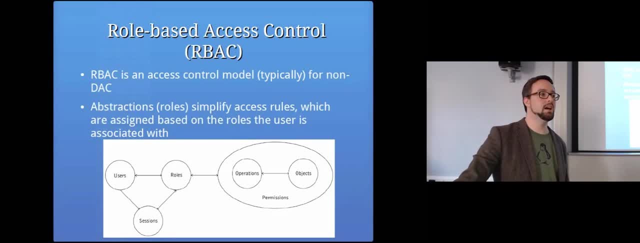 give that person all those permissions. we just have a role that they're allowed to assume at certain times, and maybe the same person has multiple roles that they can activate at various points. so, rather than just giving that person always access to everything because they're a manager, they might also have the role of being an employee, which gives them the opportunity to accept. 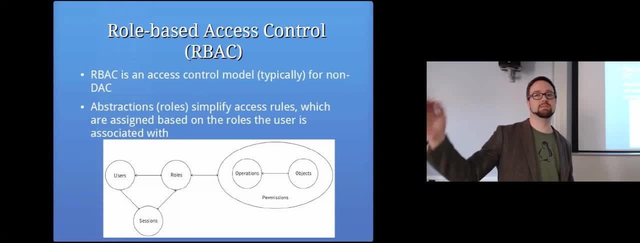 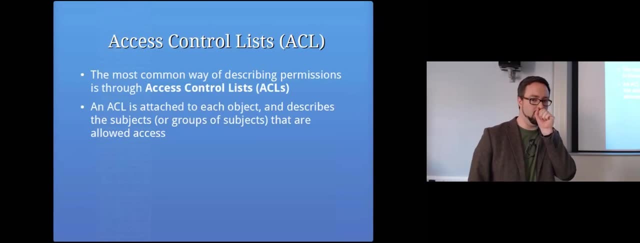 which gives them a basic amount of access and then, every now and then, they can escalate to being a manager and then they get these extra permissions. so that's what role-based access control is. so I said we were going to come back to that access control matrix and this is where I will. so an access control list. 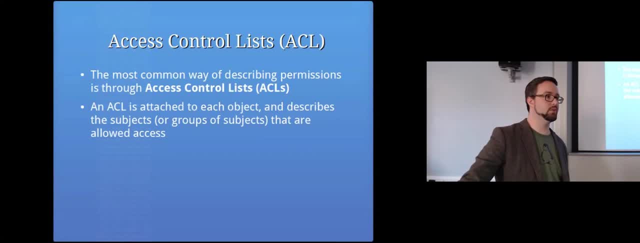 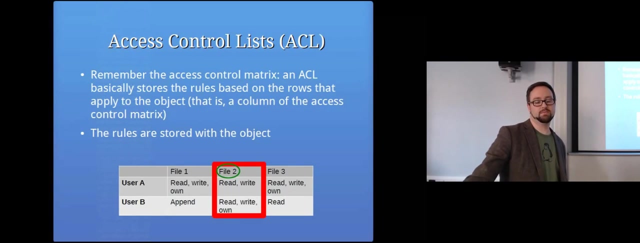 is the most common way of describing permissions on a computer system. so an access control list, or an ACL, is attached to each object, and then it describes the subjects that are allowed access. so so it's like this, so you can see this diagram here. this is the original diagram we had, but now attached. 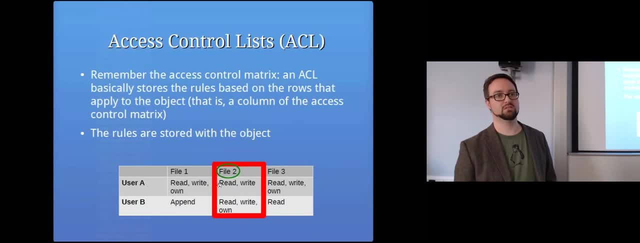 to each file is a list of all the Commission's for all the users on that system. so it basically stores all the rules for that specific file at the attached to each file. so that's the way that Windows and Linux works. so, and in slightly different ways, but similar. so on Windows they have a full access. 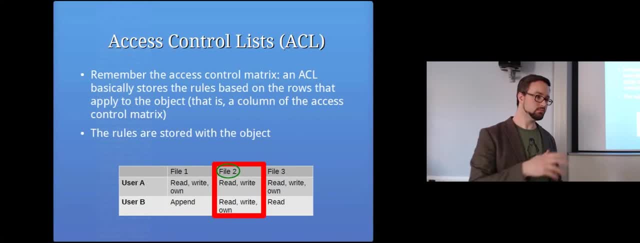 control list associated with every single file on the system. if you go into security properties for that file, you can see the list of all of the users and that are allowed to access that file. on Linux it's a slightly simplified version of that. where you it simplifies the. 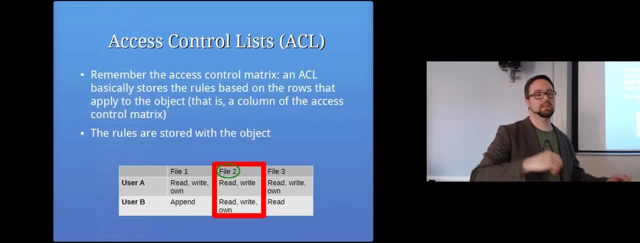 permissions that are allowed to access that file. so that's the way that the system is. it simplifies the permissions that are allowed to access that file. so that's the way that the down to the owner of the file, everyone in a specific group that the file has. 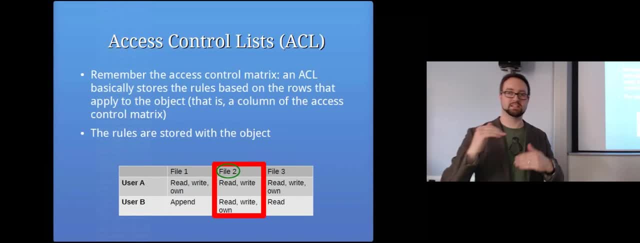 down to the owner of the file, everyone in a specific group that the file has associated with it and everyone else on the entire system. so rather than a list of every single independent user and system, it kind of groups people together into these categories. that's this the typical Unix were doing things, but you. 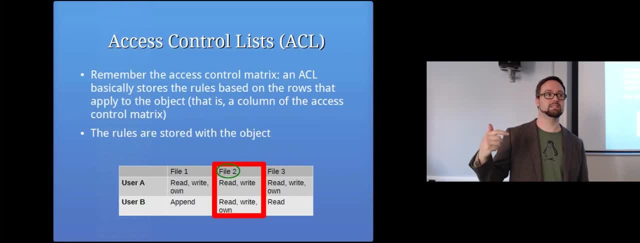 know it's not. Linux has lots of extra security features in addition to that basic way of applying the system. so that's the way that the system is way of doing things, the unix way, and we'll come back to that. so basically the idea is, with an 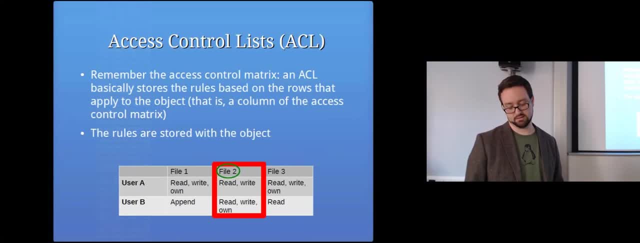 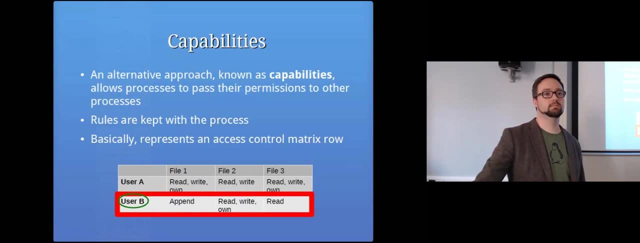 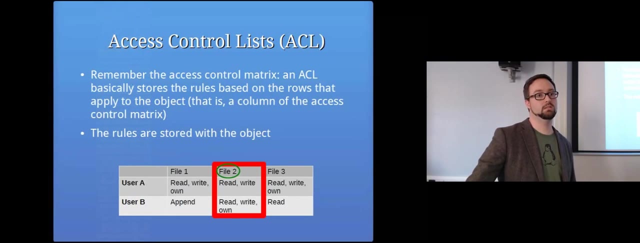 ackle. the rules are stored with the object. so that's important capabilities. yeah, sorry whether ncls, especially if you try to edit a file- this is access tonight because of the acl. yeah, and you actually have to change this thing. you can actually write and you can actually. 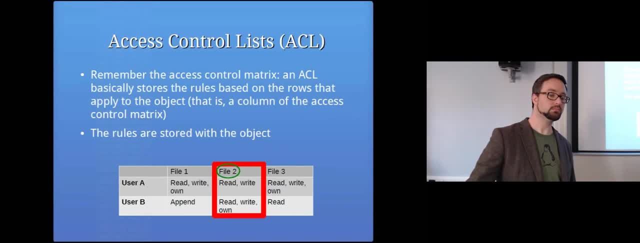 depend on the file. say, i'm on this drive, i'm about to write to it. you know, when you change it, sometimes it still guides your access to it. um well, no, if you change the permissions in theory- and i'm not advocating the fact that windows does security perfectly- 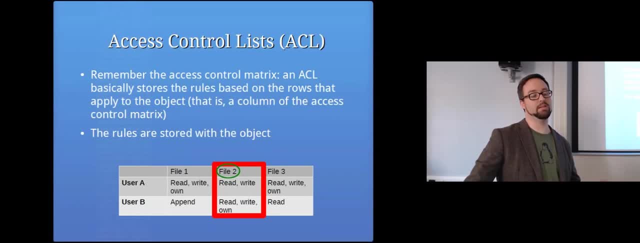 but if it's working properly, it well. there might be multiple layers of security things going on, but just looking at that one specific layer over at the ackles, because windows, uh, inherits permissions from folders and things like that above it. but but generally the permissions on an individual file should specify who can access that file and if you own that file you can change. 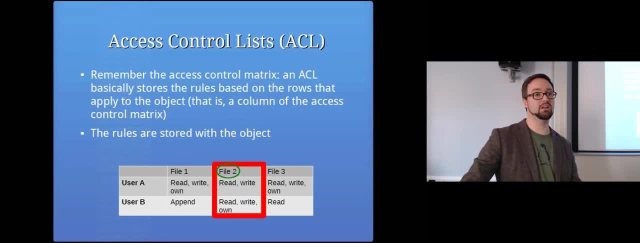 those permissions. if you don't, you need to be an administrator or the person who owns that file to change those submissions, but you can- um, yeah, it should work as it's supposed to. so you can say, if you're not allowed access to it, if actually using your computer. 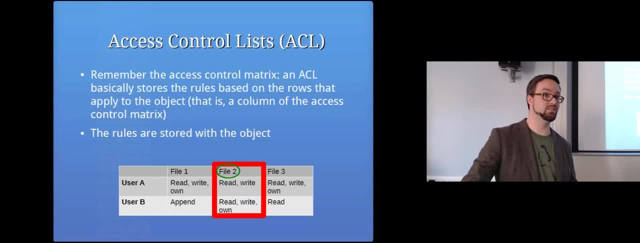 and you've got multiple users sharing that computer, they should have independent user accounts. and then, if you've got certain files that you want everyone to be able to use on that computer, you would set the permission so that everyone's allowed to access it or certain users are allowed. 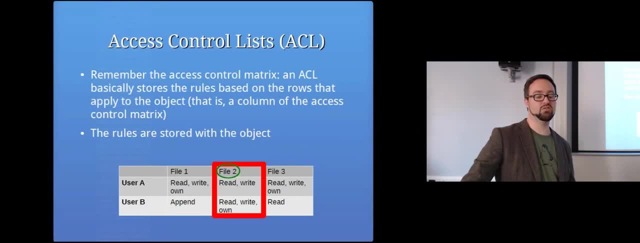 to access it. um, it's not good practice to have a shared computer with everyone using one account. um, it's just. it's good to have separate accounts for everyone, even just so that they don't set you don't have to look at desktop backgrounds that you don't like. 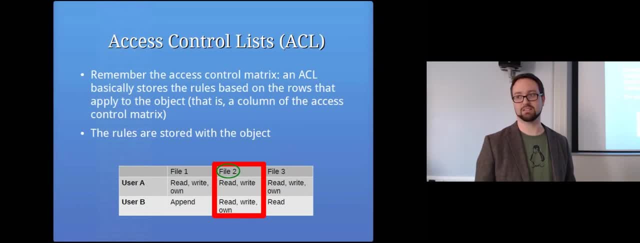 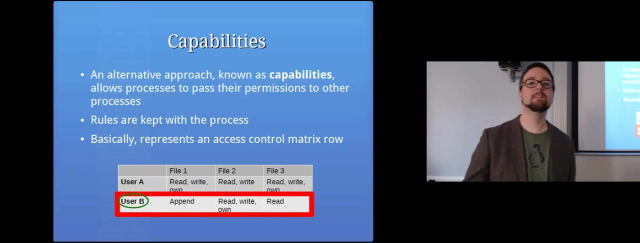 no, um, but you know, from a security perspective, you should be using it correctly. um, does that answer your question? sort of yeah, so i'm not into it. yeah, yeah, okay, that's fine. uh, so capabilities is an alternative approach. so, instead of attaching all of the information about who's allowed to do what to the 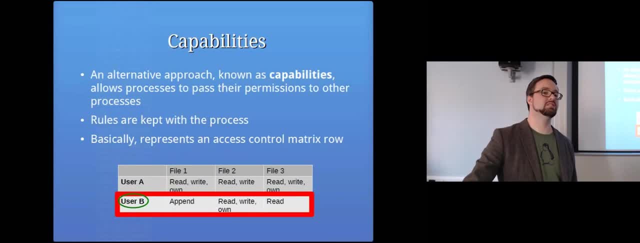 to the objects, we instead attach that information to the subject. so, basically, we keep the rules with the processes. so if, for example, um going going back to our not that inventive analogy of having physical files with things attached to them, if i had a printout of something and i stapled to it a list of 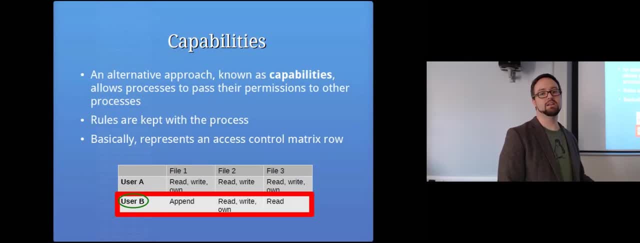 all the users that are allowed to read that file. that's an access control list. if, instead, i give you on your name badge a thing that you can click onto it, that has a list of files you're allowed to access, we're now talking about capabilities, so it's information that's kept with the, with the. 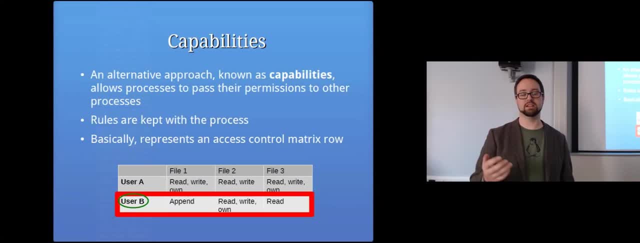 the actual subjects of the system, and obviously you need a way of obtaining the actual capabilities. but there's, there will be some mechanism for you to get proof, a token that says you're allowed to access something, and then when you go to access it, you'll you'll be allowed to access it. so that's. 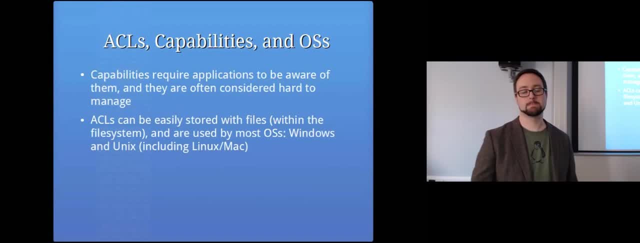 what a capability is what i was. uh, is it okay to, from a security perspective, um, to run as an administrator if there's only one account, or should you have an administration account and then you should never, ever, ever run as an administrator? you should not log in as an administrator or a root user ever, because it's too. 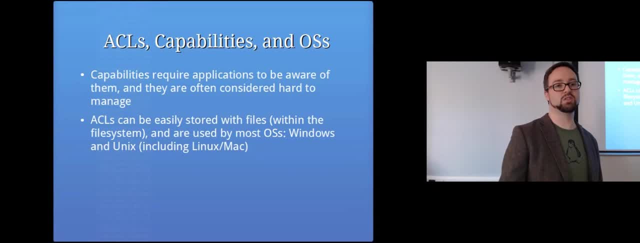 well, i can list how many reasons do you want? i'll give you two main ones- is that you can make mistakes that are fatal- hopefully not physically fatal, but you know you can make you accidentally type in a command and you've just wiped the entire computer like you've deleted the operating system. 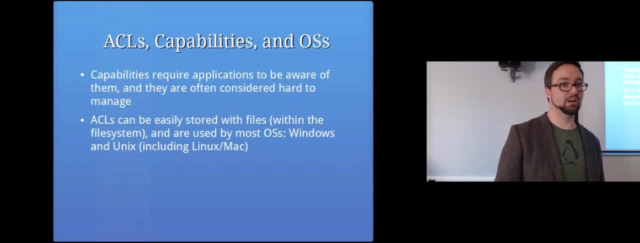 well, there's been various problems with that on on windows as well, but it but yeah, that's still- at least that's a level where you actually need to authenticate, like if you have a linux or a unix system, you should be logged in, not as root, and then you should have. 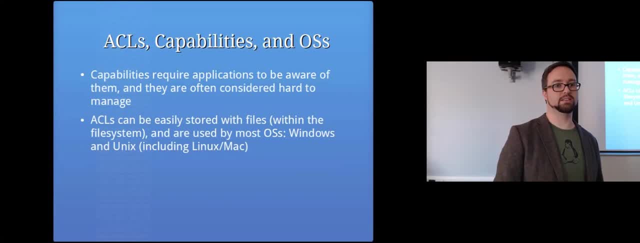 to elevate your privileges to do the things that are important. so you type the root password to prove that you're allowed to do certain things, or, if it's an ubuntu system, you have the permission to basically use your own password to do root things, which is similar. 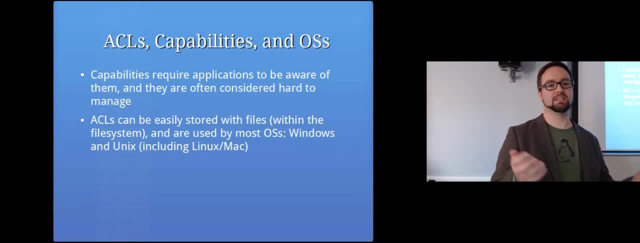 to a windows like user account control, where you can like specifically escalate to do certain things. so the windows security system tries to have that balance where you might be an administrator but you can't just delete things without clicking something on the screen. but there have been various problems with that mechanism in the past, so it's not. it's not. 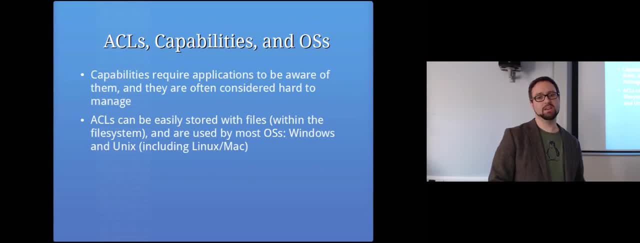 perfect, but it's better than nothing. um? so, if we're talking about capabilities versus ackles, capabilities require applications to be aware of them, and they're they can well. they're considered to be hard to manage, uh, although some people in security committee will strongly argue the opposite. 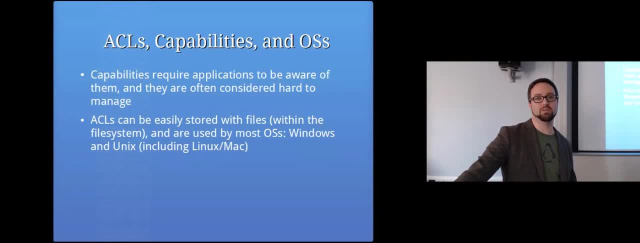 but access controllers, uh, just easy in general, because we just store them with the files. so it's very straightforward, basically, and they're stored within the file system and that's the way that most operating operating systems do things. so, on windows and unix, which includes linux and mac, we use ackles for